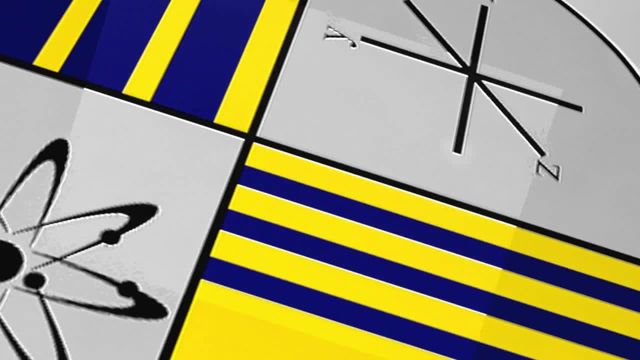 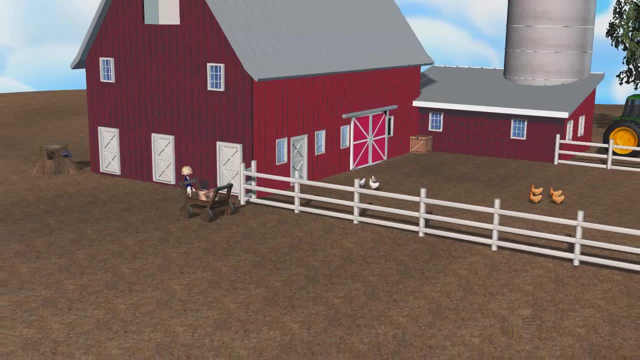 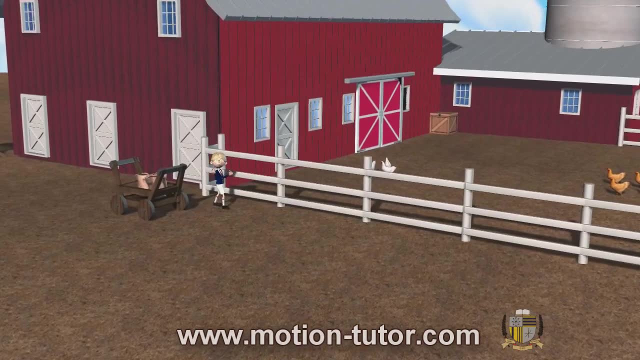 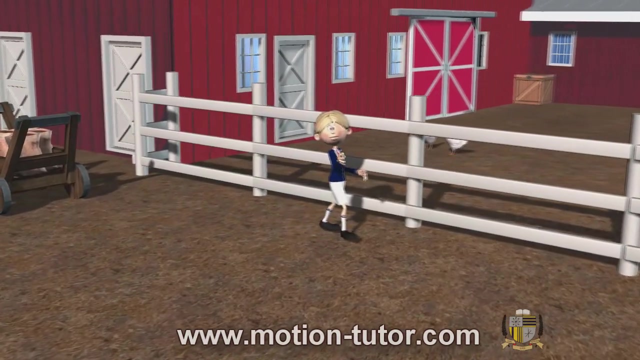 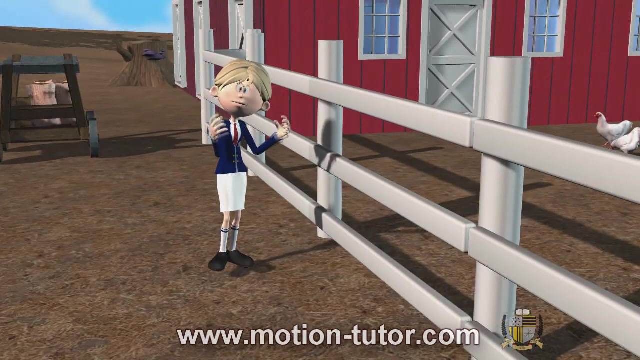 Hey everyone, Welcome to EmotionTutorcom video lesson. This lesson will be understanding addition stories. So this is addition, but we're going to dig a little deeper and try to understand what's going on with some addition stories. I will be telling you Here I am on the beautiful 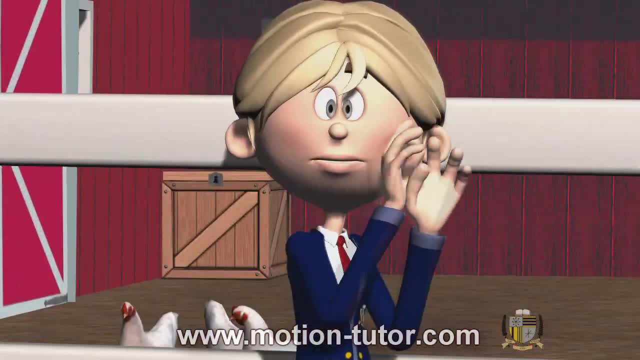 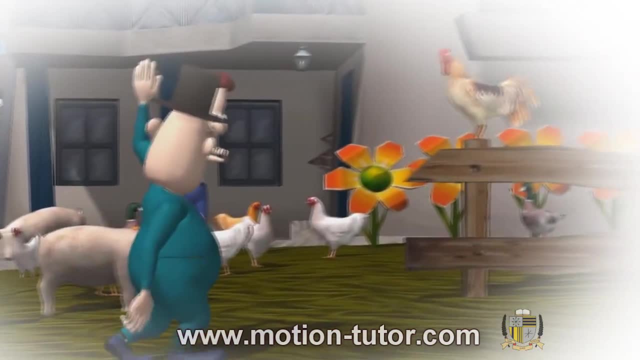 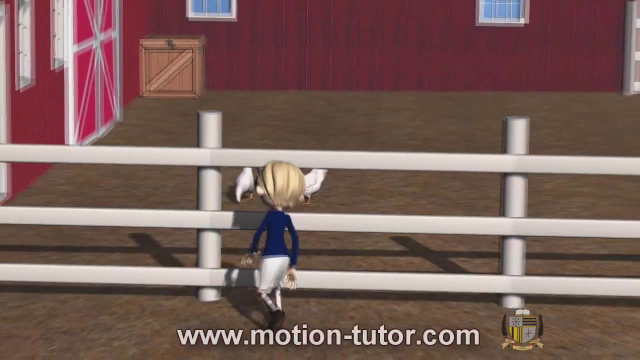 Bob's farm. Hey, just a little side note, This is the farm where the guy in the story Bad Neighbors called to get all those animals for his neighbor. Yeah, this is the farm he called. Anyway, let's get to the addition stories. 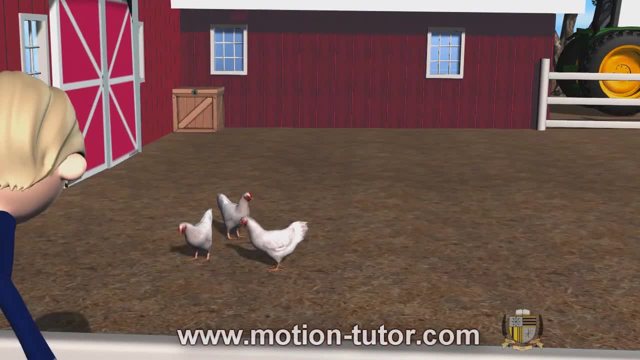 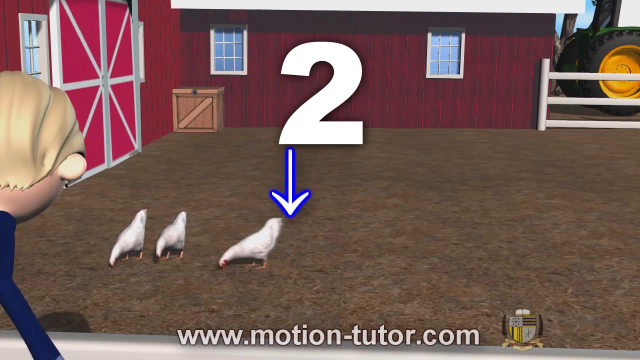 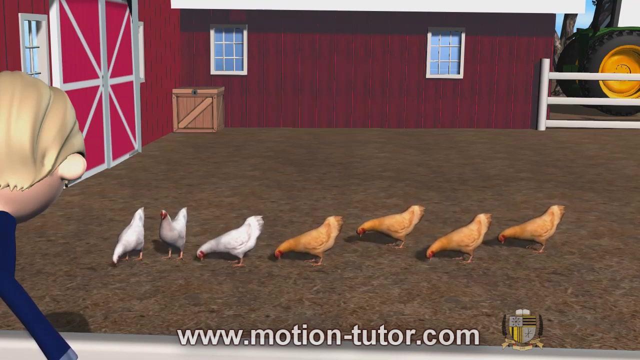 All right. I see three white chickens eating from the ground. Let's count them One, two, three. In comes four brown chickens. Let's count them One, two, three, four. All together, how many chickens are eating from the ground? 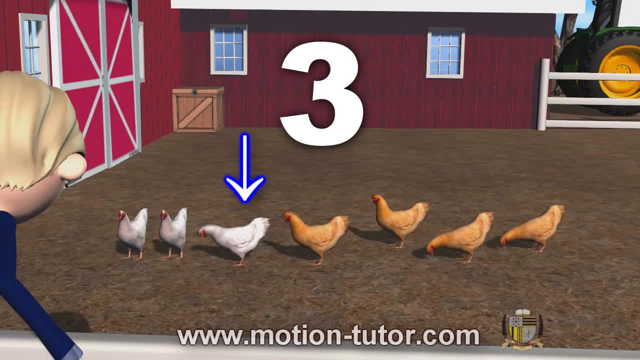 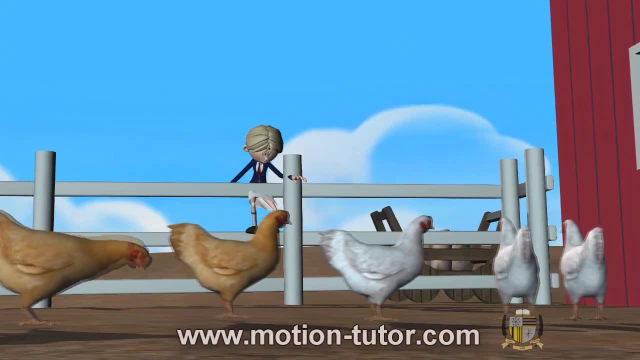 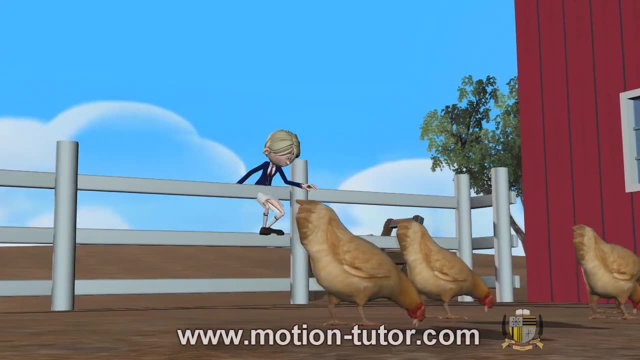 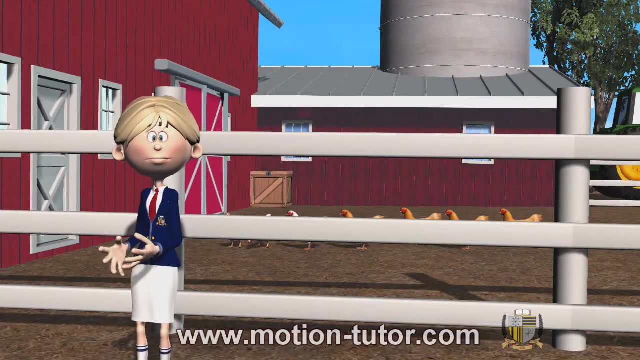 One, two, three, four, five, six, seven. So all together there are seven chickens eating from the ground. Now let's look back at this story. How many chickens were there at the start of the story? Do you remember? Three chickens. 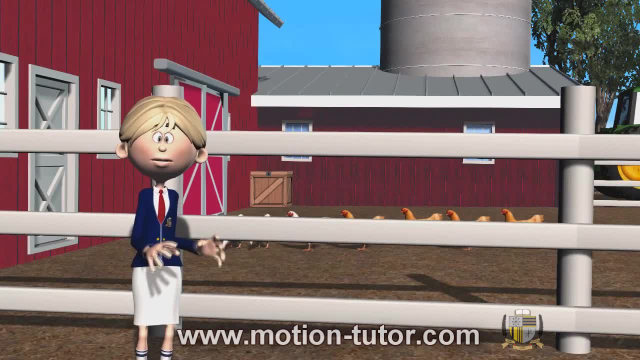 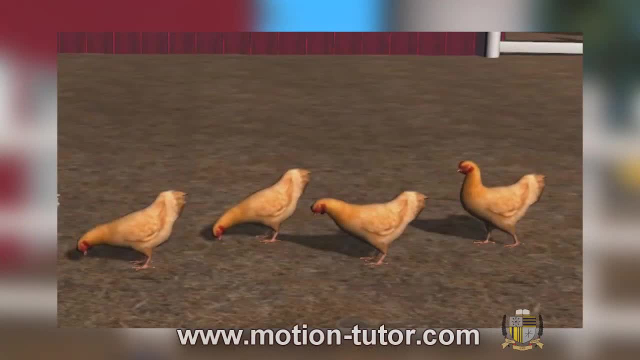 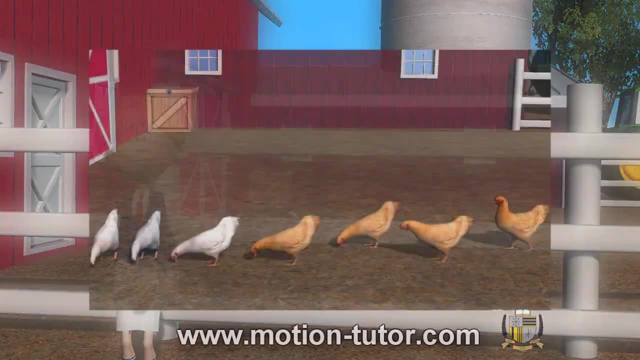 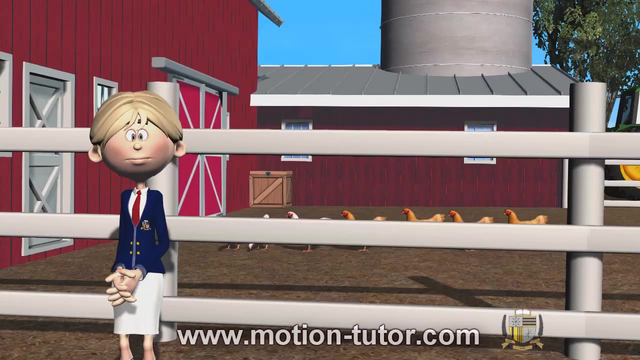 One, two, three. How many chickens joined them? Do you remember? Four, One, two, three, four, And how many are all together? Seven, One, two, three, four, five, six, seven. Moving on to this truck over here. 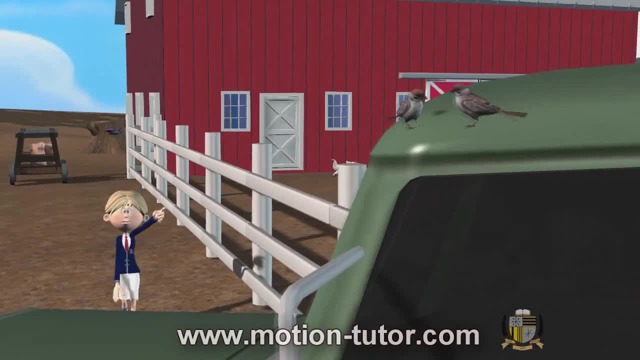 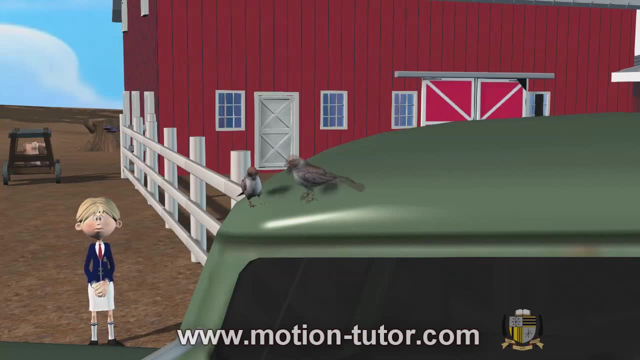 We see two birds on top of this truck. Let's count: One, two, Three blue birds join the other two on top of the truck. One, two, three. How many birds are there on top of the truck? One, two, three, four, five? 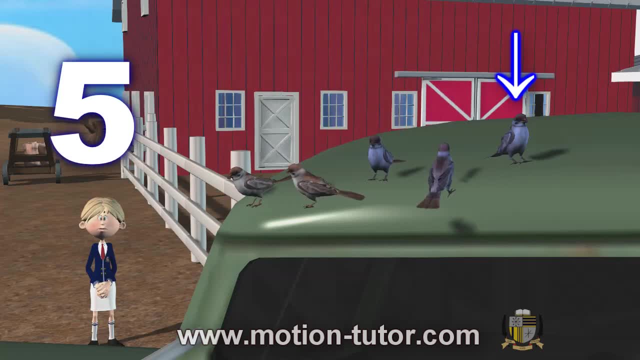 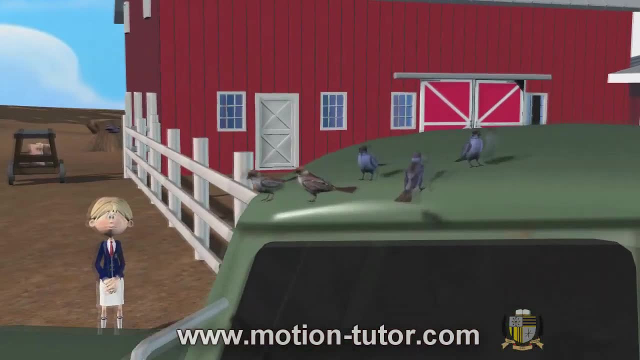 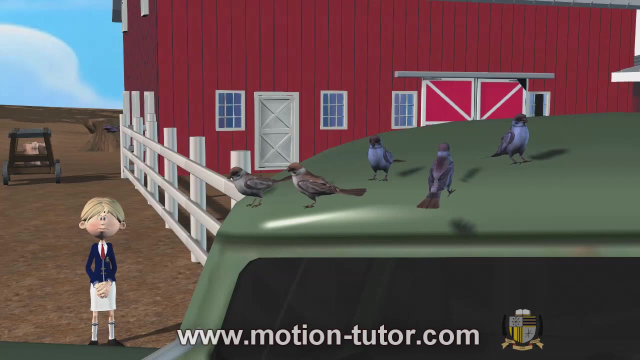 Two, three and one, Two and one, Two and one. There are five birds all together, and they're all on top of this truck. So now let's look back at that story and think how many birds were there at the start of. 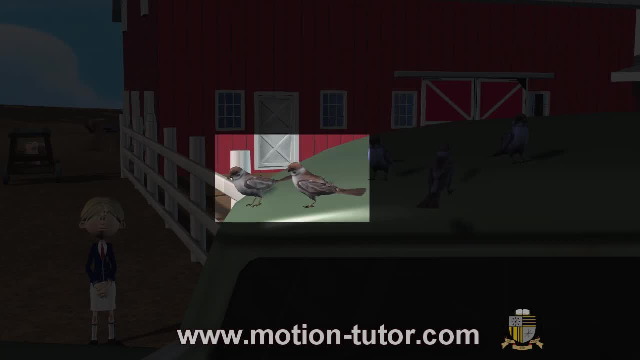 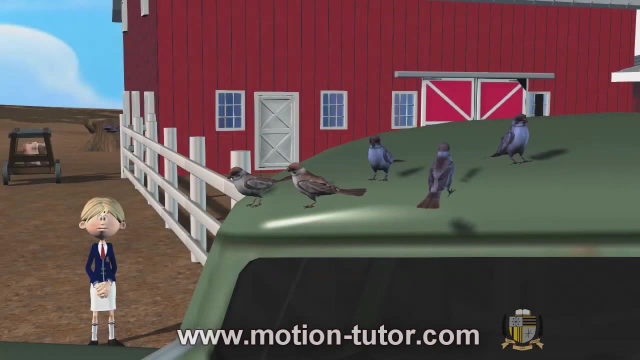 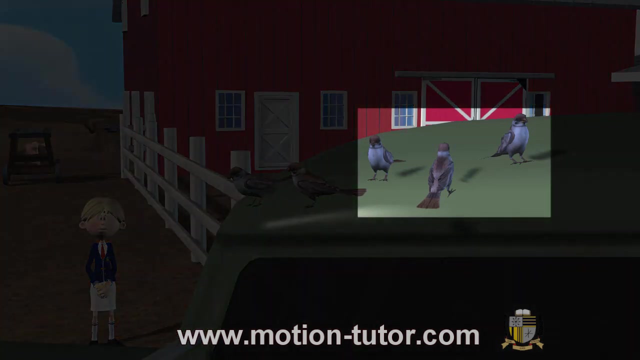 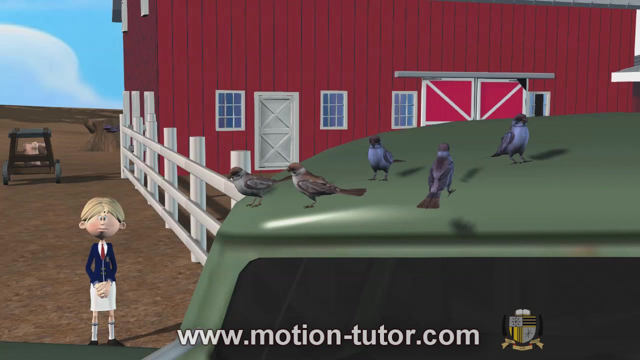 that story. There were two birds. remember one, two, And how many birds decide to fly in and join those two? Remember the blue birds? there were three. one, two, three, And how many birds all together? One, two, three, four, five, five birds all together? 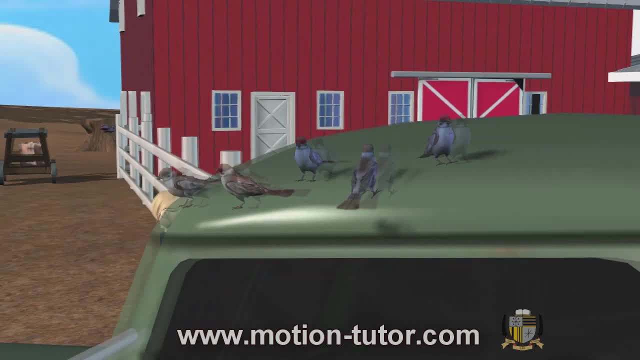 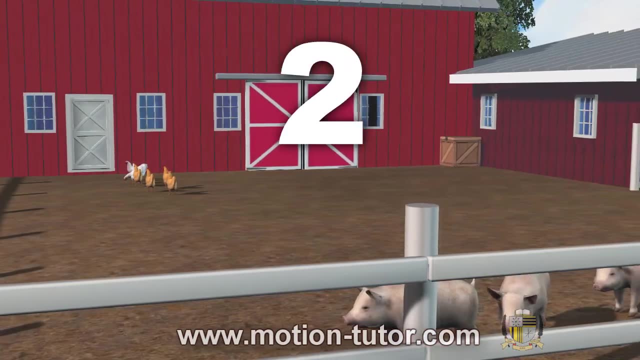 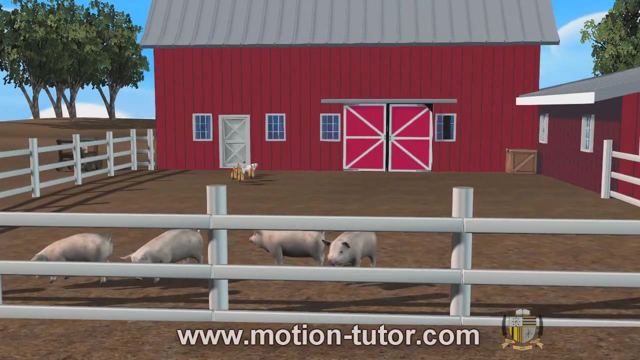 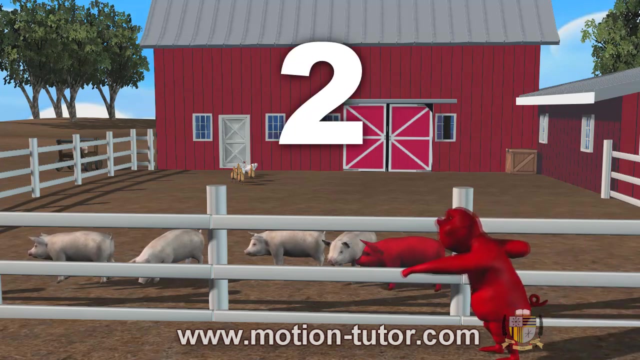 All right. moving on to our last example, I see four pigs in the yard: One, two, three, four, five. One, two, three, four. Then two red pigs decide to join the four pigs. one, two. 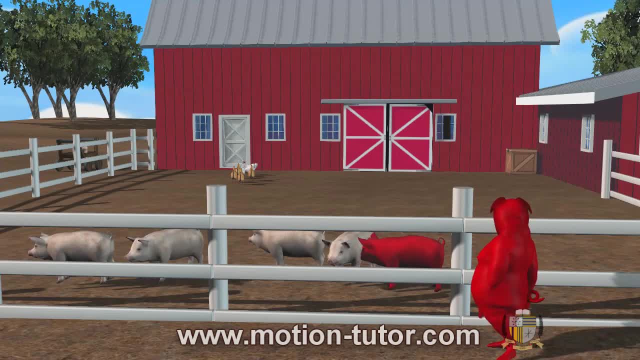 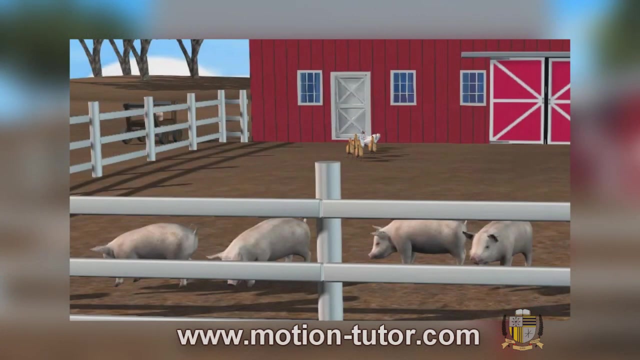 How many pigs are there all together? One, two, three, four, five, six. So there's six pigs all together. So now let's take a look at that story. How many pigs were at the start of that story? remember, four pigs. one, two, three, four. 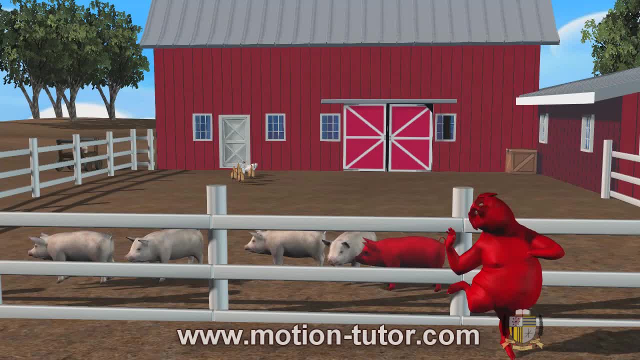 And how many pigs join those four. Remember the red pigs: one, two, And how many all together: One, two, three, four. One two, three, four. One two, three, four, five, six.